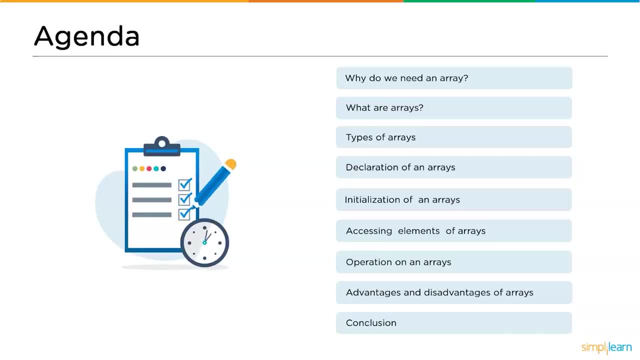 declaration of arrays, Followed by that we will learn how to initialize an array, then access the elements in an array. After that, we will understand the basic operations that can be performed on arrays. And, to wind up the session, we have the advantages and disadvantages. 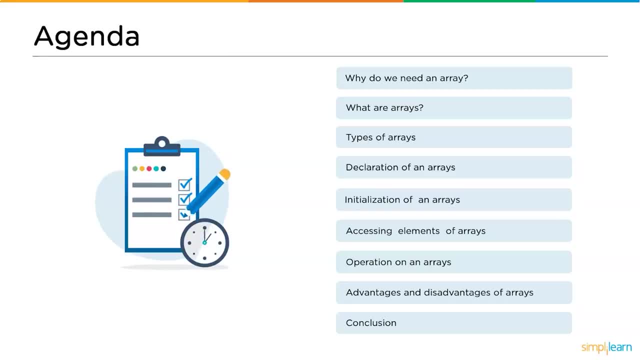 of arrays. At the end we will have some of the basic operations that can be performed on arrays And some key takeaways. I hope I made myself clear with the agenda. Now let's begin with the first topic, That is, why did we actually need an array? 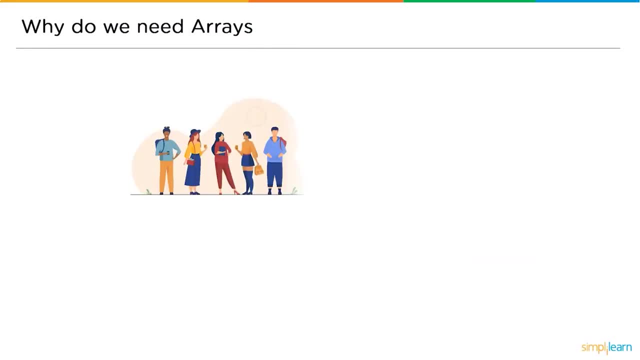 So to understand this, let's go through a simple concept. Let us imagine that we have some data and the data is related to students, right? So if we wanted to store the marks of individual students, then we had to declare a variable for each of the student. 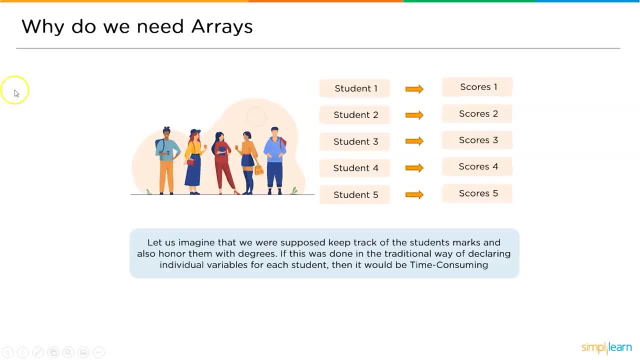 So you can see we have student 1,, student 2,, student 3,, student 4, and 5 and their individual scores. So the score 1 is assigned to student 1 and so on, with student 5 being assigned. 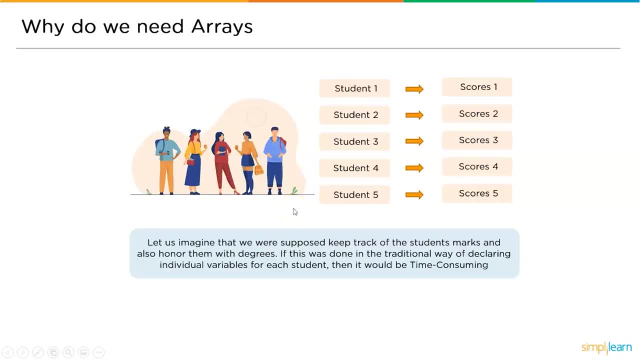 to score 5.. So in the real time this might be a little clumsy. We have here just 5 students, So that is okay. But what if we had 500 students or 5000 students? right, That might. 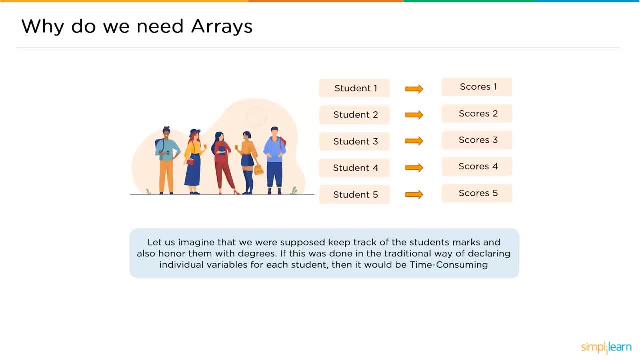 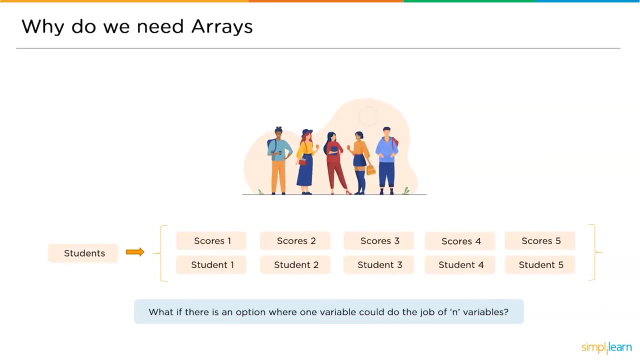 might be an issue there. we have to create some 500 or 5000 variables and it would be a little tough to handle that right. even if we wanted to apply some operations collectively on all the variables, that might be a little tedious. so what if we had one variable which could store all the 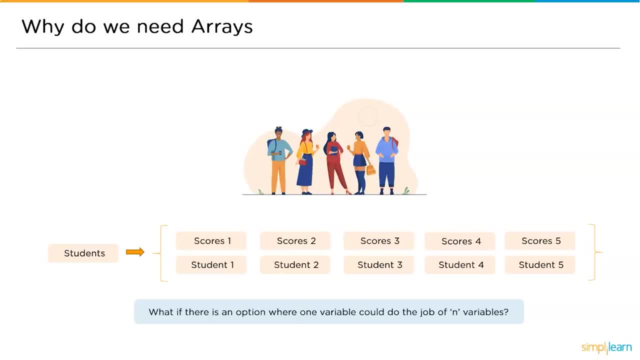 five students or 500 students, or 5000 students all together, and make it really easy for us to apply some operations collectively on all the students, right? this sounds a little bit logical. so, similarly, we do have a data structure which can do that, which can collectively store all the. 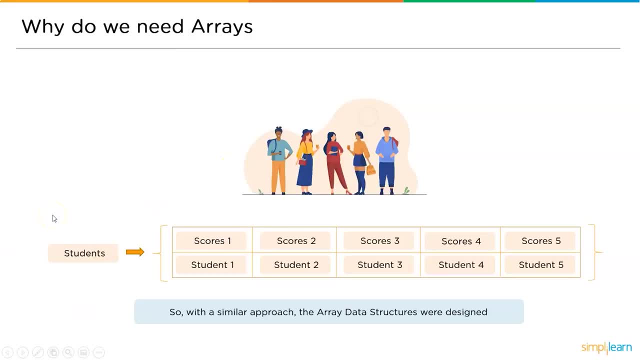 data elements in it as a single variable, and it will also help us to apply the operations which are logical or mathematical on all the variables and their values together as a whole. so that is the purpose why we had created arrays. that is the purpose why we needed arrays. so far, we have understood what was the necessity for arrays. now we will understand. 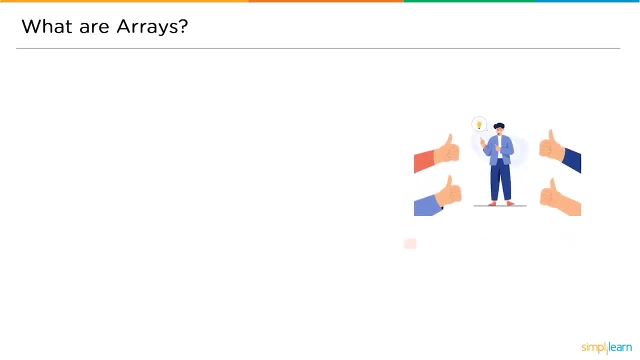 what exactly are arrays? so basically, an array is a linear data structure that stores the elements in a sequential manner, one after the other, and when you declare an array, the variables will be stored one besides the other, that is, adjacent to each other, in a sequential order. now let us 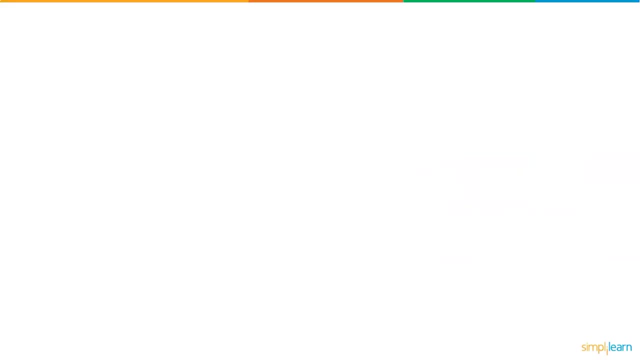 understand how the array is represented by the compiler. now the next part, that is, the memory representation of arrays. now let us imagine that we have declared an array which stores character type data. and another important point to remember about arrays: when you declare an array, it stores only a single. 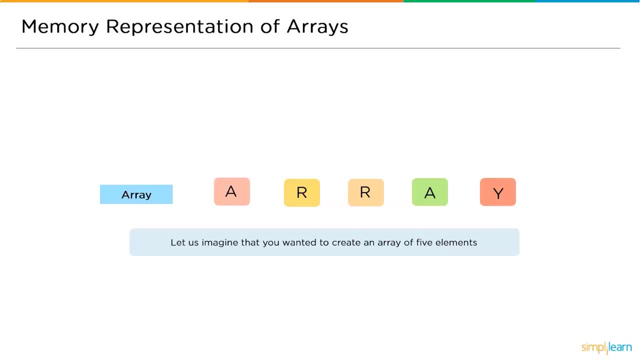 data type typed elements only, for example, here we have declared a character type array, right, so we cannot store integer type data or flow type data in it. we only have to save character type array or character type elements in this particular array. So now let us imagine that we have created an array which is of character data type. 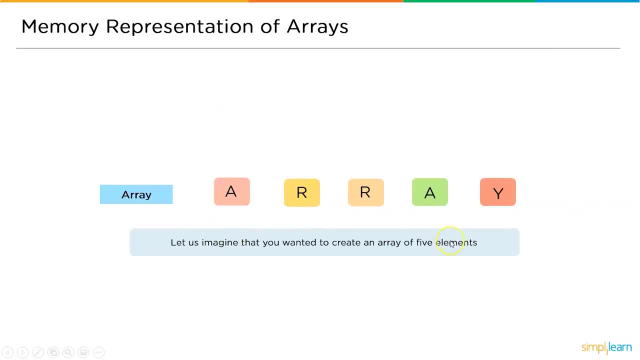 and these are the elements which are a r r a y. Now, how does the compiler represent it? in the form of memory. So when you create an array, these are formed, that is, the index, values and the address. So basically, compiler will select a block of. 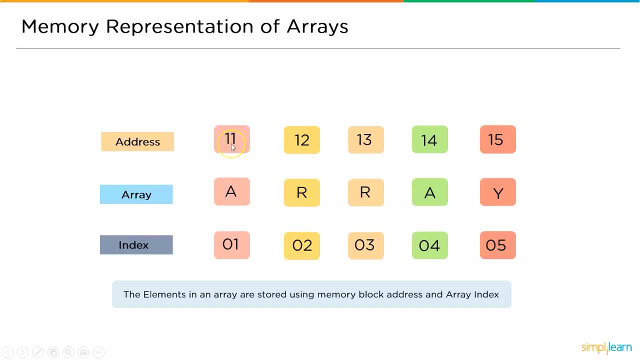 memory and it has addresses to that block and it can be anything. Right here we have 11,, 12,, 13,, 14 and 15, and in real time it might be 1001, 1002, 1003, 1004, 1005.. The main motto is: assign a. 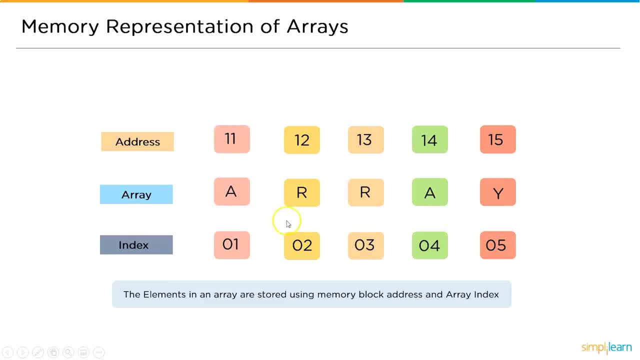 sequential block of memory and this is the array, and the elements are a, r, r, a, y, and this particular one, which is the last one, is the index of the array, that is, the position of the array for user. So, using this index, 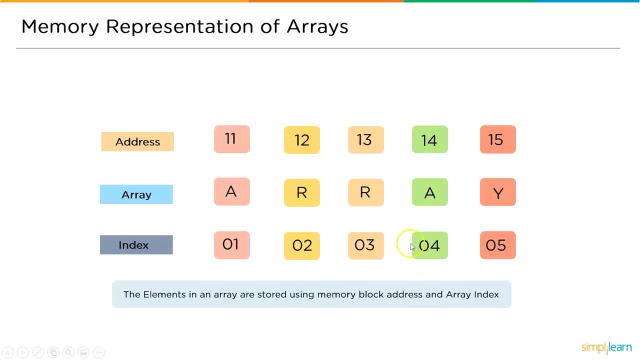 you can access the elements in the array. More on that in the accessing part. So let us imagine that we wanted to access the element r. So how to access it? We might not know the address right. In that instance we will use the index. this is for r reference. 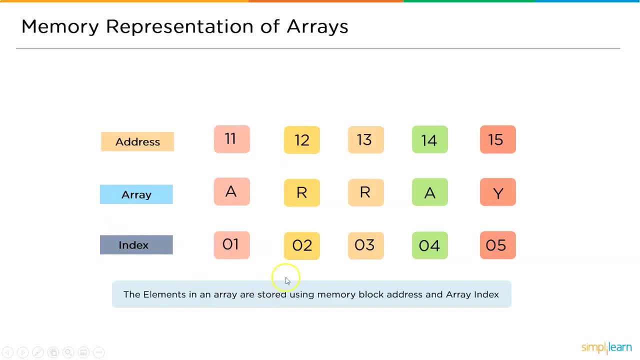 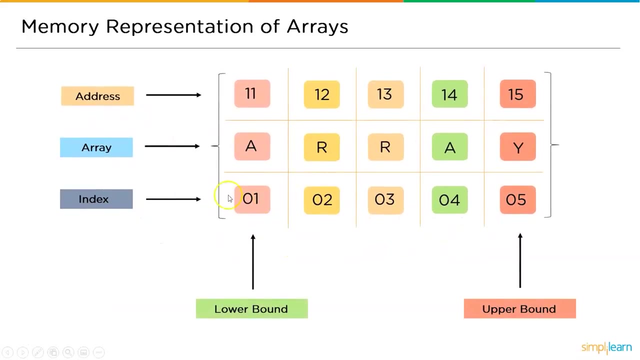 So we will tell: I want the element from array index number two, and then we will have the arr r element. So in the practical form this is how we use the index. Now let us continue with the lower bound and the upper bound. So the first initial location is called as the lower bound, and at the last or 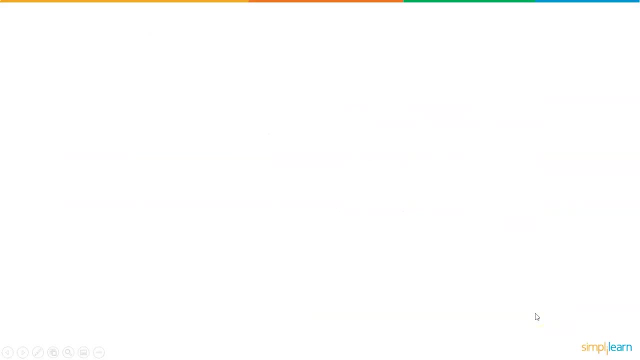 the max value of the array is called as the upper bound. Now let us jump into the next topic, where we will understand the different types of arrays. So these are the different types of arrays: One-dimensional arrays and multi-dimensional arrays. In multi-dimensional arrays we have 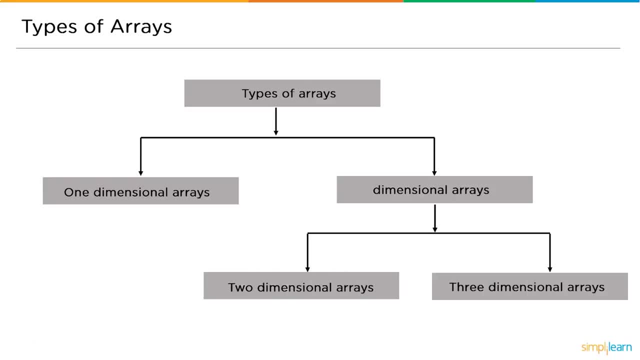 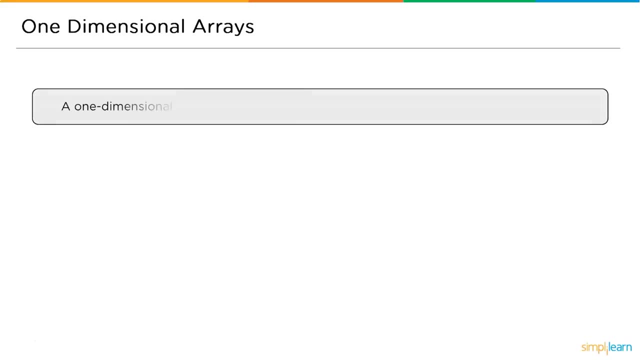 two more types, that is, two-dimensional arrays and three-dimensional arrays. So how are arrays different from each other, Right? So the first one we will deal with. the first one, that is the one-dimensional array. Now, how is an array declared as one-dimensional? 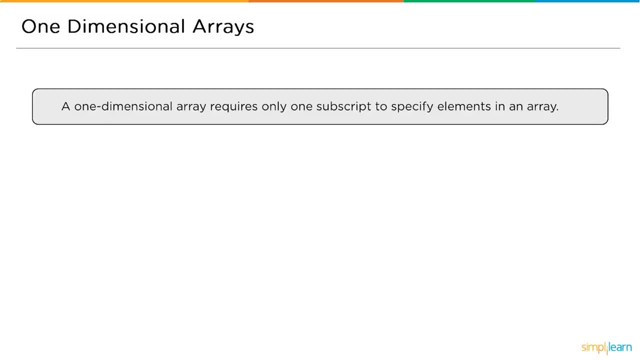 For that we need subscript. So one-dimensional array requires only one subscript to specify the number of elements in an array. So how is it actually represented? So here you can see an example right on my screen. So here is how a one-dimensional array looks like. 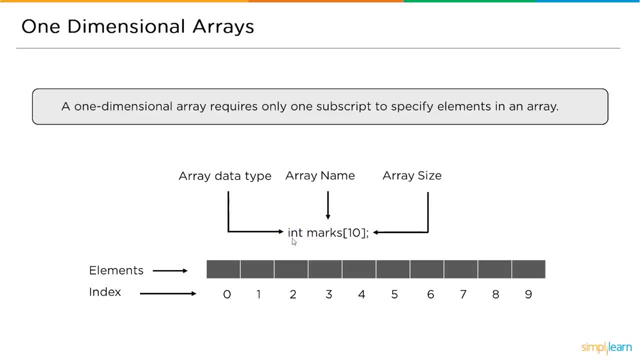 So here we have the data type, that is integer data type and marks is the name of the array and this is the size of the array and here the elements will be stored and here it is the index value of the array, and remember, the index value of array always starts from zero. 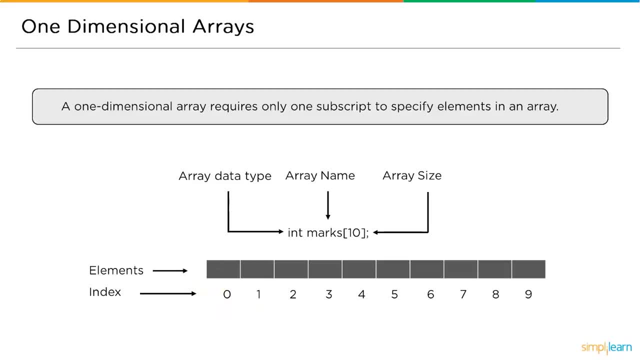 In the previous example. that was only for basic understanding, so I just started that with one. In the practical way, the array index always starts from zero, So, followed by the one-dimensional array, we will deal with the multi-dimensional arrays. 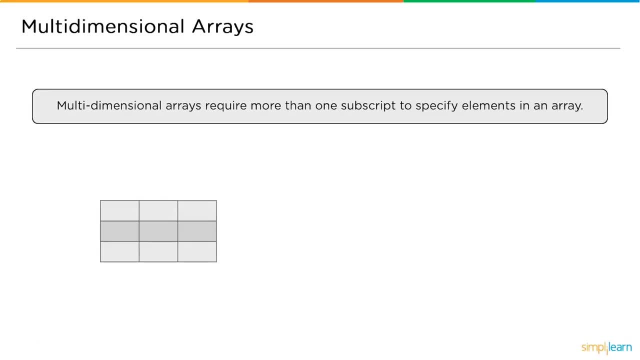 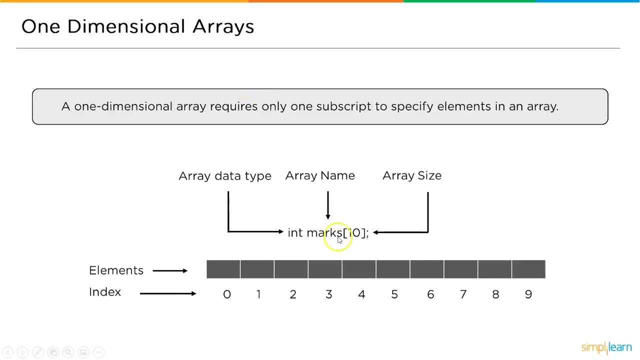 In that we have the following: The first one is the two-dimensional array and the second one is the three-dimensional array. In the multi-dimensional arrays we require more than one subscript. In the previous example we had one-dimensional array, So this subscript is just one. 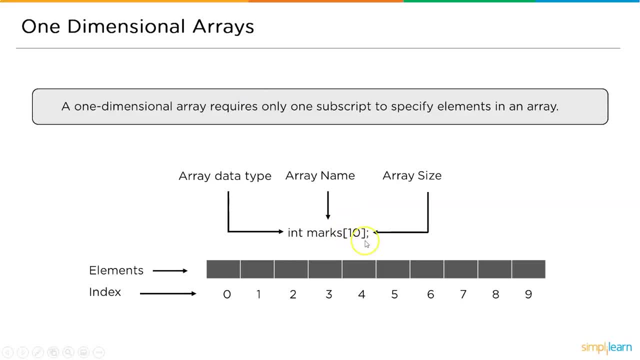 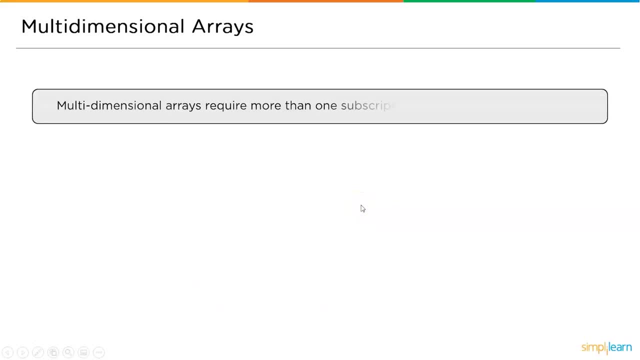 one that is 10 columns, right? So we just had one single row and 10 different columns. but in the multi-dimensional arrays we need multiple rows and multiple columns, right, So we need two subscripts for two-dimensional array and more than two subscripts for three-dimensional. 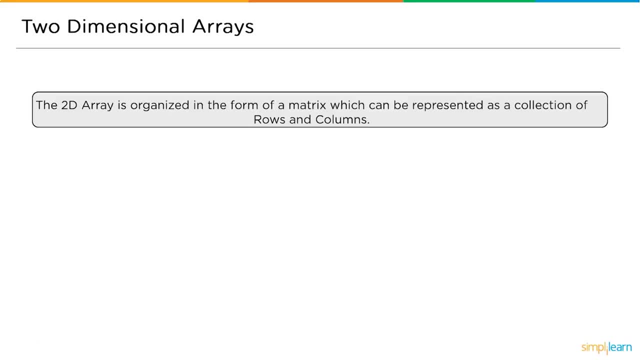 arrays. So first we have the two-dimensional arrays. The 2D array is organized in the form of a matrix which can be represented as a collection of rows and columns. So here is the example. As you can see on my screen, we have three columns and three rows and we have two. 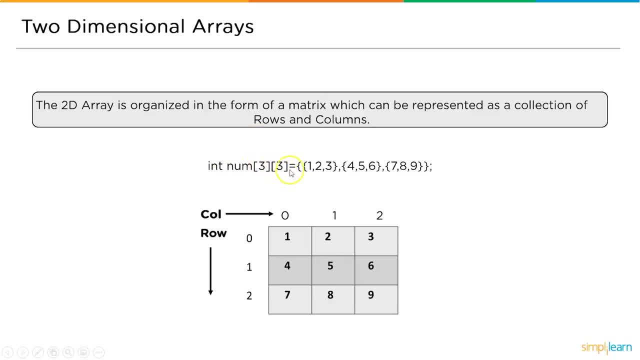 subscripts that define the number of rows and the number of columns and the elements in each and every row. So the 1, 2, 3 confines the first row, 4, 5, 6 confines the second row, and 7, 8,. 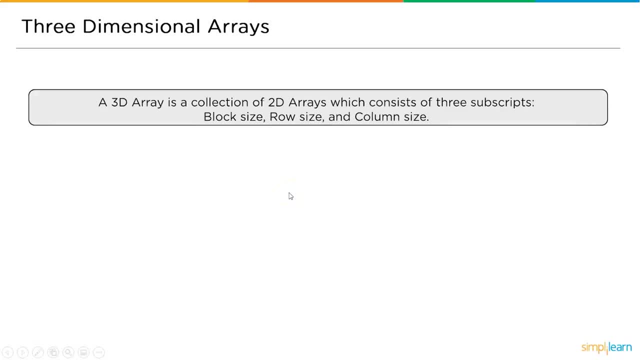 9 will be the third row Now. similarly, we have three-dimensional arrays. A 3D array is a three-dimensional array, So we need three-dimensional arrays. So an array is a collection of 2D arrays which consists of three subscripts. block size: 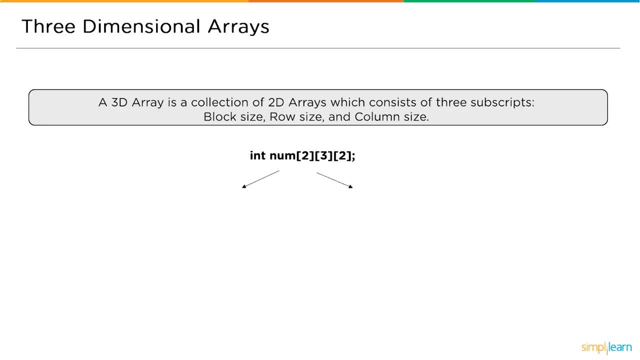 row size and column size. So here we have an example for that. So we have three subscripts, that is, the first one is block size, the second one is the row number and the third one is column number. So this happens to be the first block. 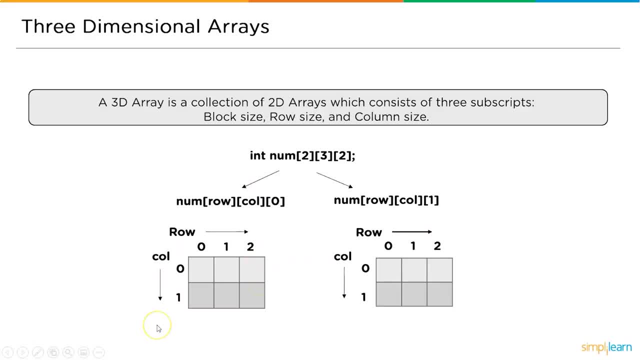 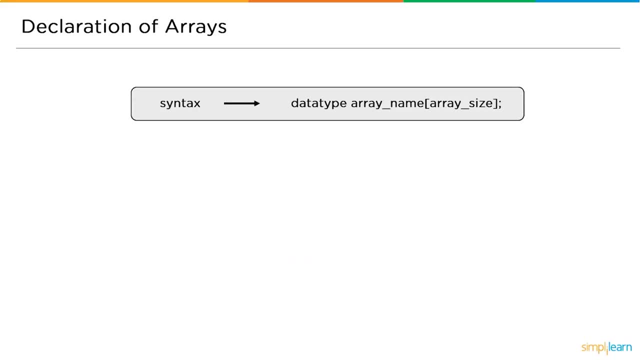 this happens to be the second block, and this is how a three-dimensional array can be represented. Now we have the next stage, where we will understand how to declare the arrays, and the syntax is right on my screen. You need to specify the data type of the array. 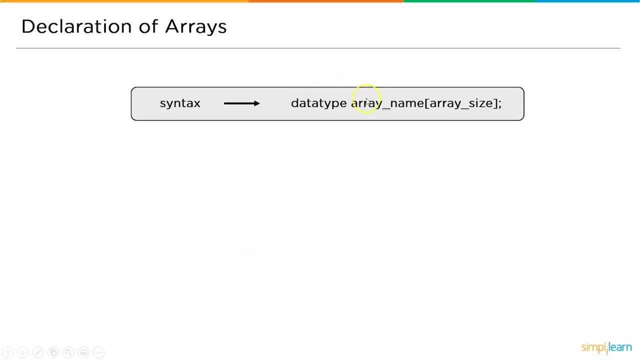 which is integer, float or character, any selection which you make- Followed by that, you need to select an array name for your array and inside that you need to declare the array size, and sometimes you can also eliminate the array size if you wanted to have a dynamic array. 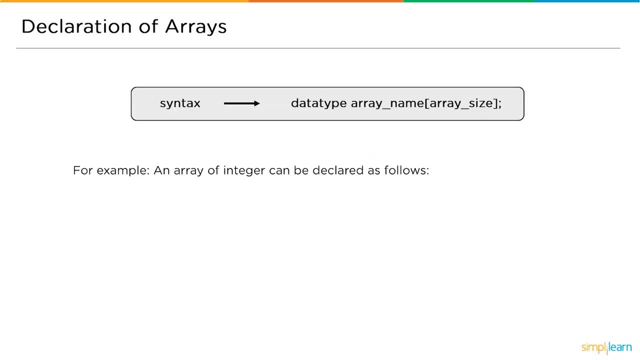 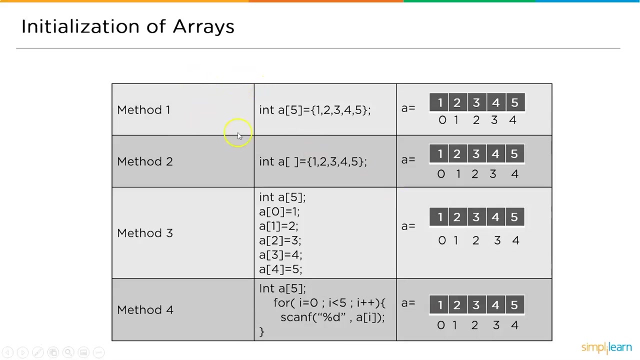 and here is an example for that. You have integer data type- name of the array is an example and the array size is 6.. So the compiler will allocate continuous memory block of six integer type blocks. So these are the few more methods to initialize the array. So here you can see. 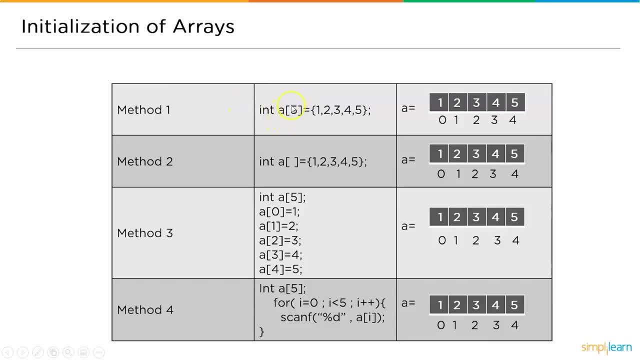 integer data type. array name is A element, size is 5 and we have 5 elements. The method to initialize the array is as shown in the example is: remember i have said you can eliminate the size of the array, right, so here you can use this way as: 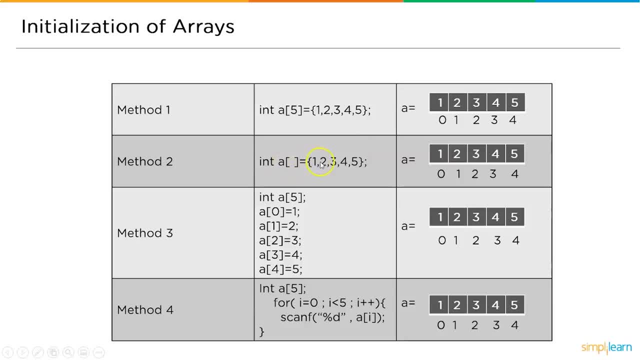 well, integer, data type, array, name a and no size here and you can directly declare the elements and the method. third, so here you have the name of the array, size of the array and you are allocating the elements to the individual memory locations. this is also another method to initialize array. 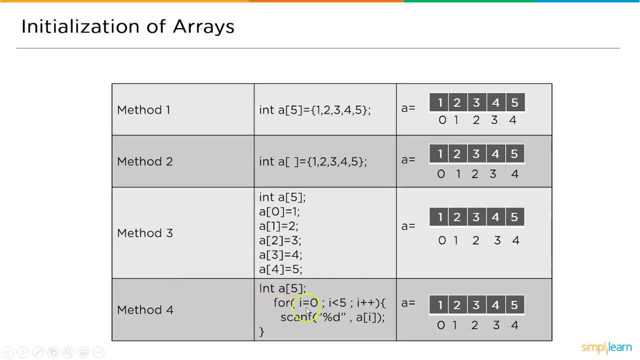 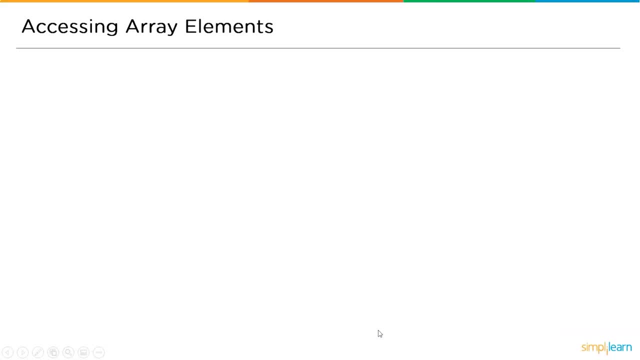 and method 4 is using a for loop. you can just initialize a for loop and the i value will be stored in the array locations, starting from zero. now let us understand how to access the elements in an array. so, to access the elements in an array, you need to specify the name of the array and 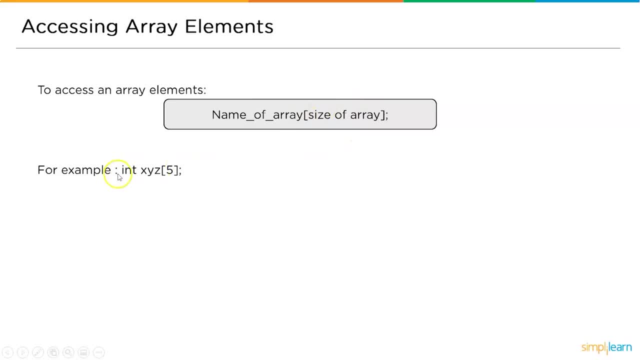 memory block where you have that element that you want to access. so here we have an example which is integer data type, name of the array is xyz and the element we wanted to access is 5.. so here we have an example that is integer type array, array name is xyz and it has the size 5.. 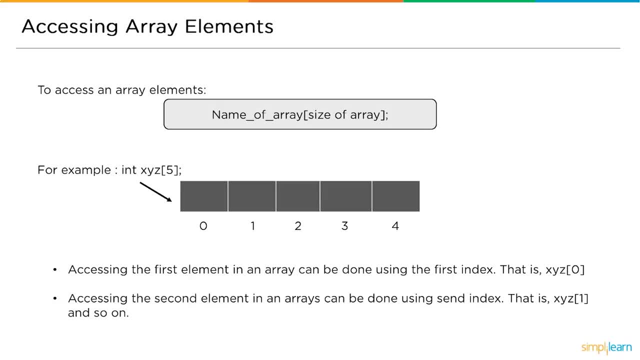 and now we wanted to access the first element in an array. that can be done using the first index, that is, xyz of 0 index, that is the first element, and accessing the second element, and so on. xyz of 1 will be the second element, xyz of 2.. 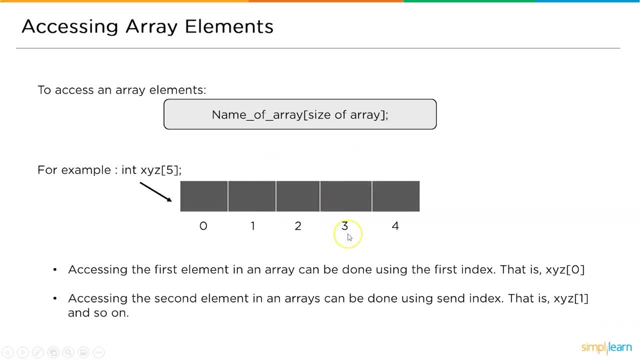 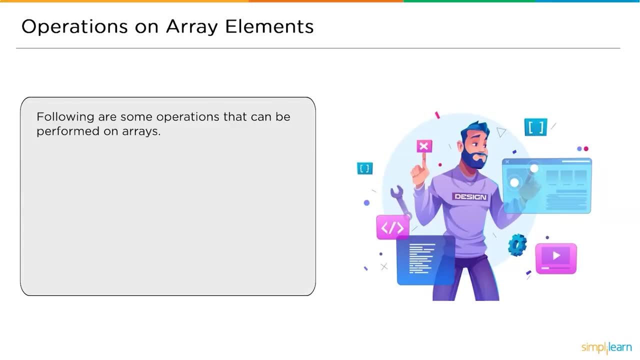 so we will even add alpha depth in the array. that is like right now, which is the first element of our array, or we can say alpha depth, the second element, xyz of 2. right, and now we can see that from the array that we wanted to access, elements 1,2,3,4 will be the 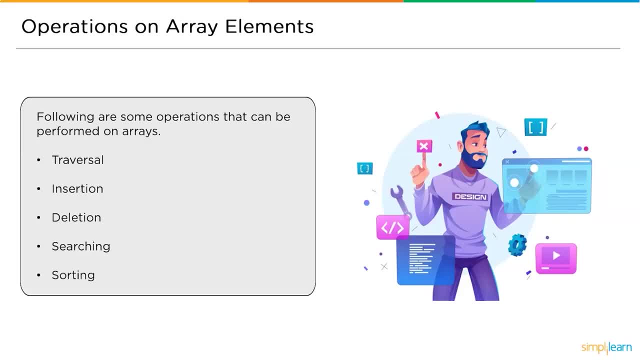 third and fourth and fifth elements. now let us understand some basic operations that can be performed on the array elements. so the following are the operations that can be performed on the array elements, that is, the traversal insertion, deletion, searching and sorting from an array, searching for an element in an array and sorting the complete. 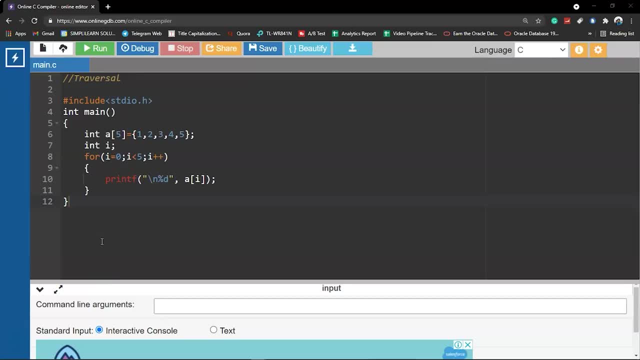 array. so at first we'll carry out the traversal operation. so here we have an array that is a of 5 and the elements are 1, 2, 3, 4 & 5. now we are going to use a for loop to traverse through this array and print all the elements sequentially. 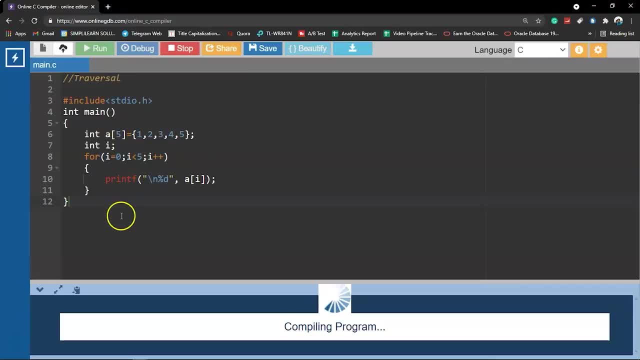 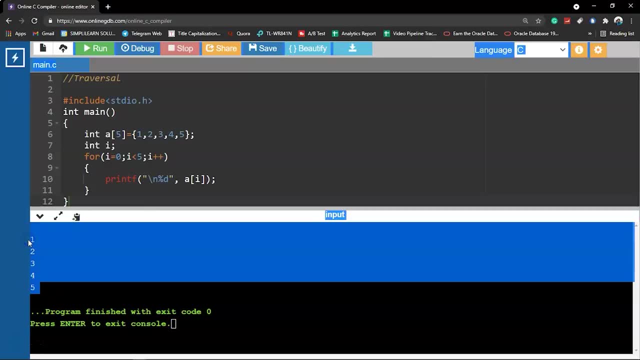 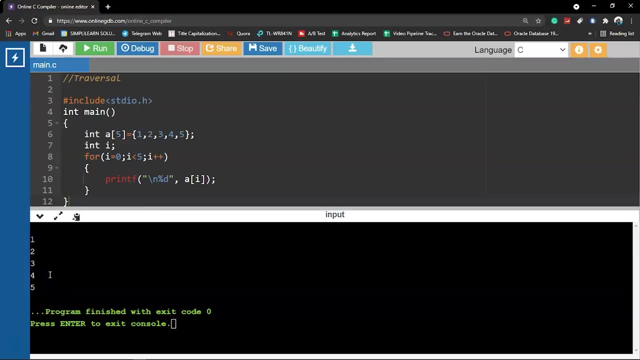 now let us execute this code and see the output. so, as you can see, the code got successfully executed and the elements, that is, 1, 2, 3, 4 & 5 from the array a are printed sequentially. now, moving ahead, we'll try to execute some examples based on insertion of element into the array. 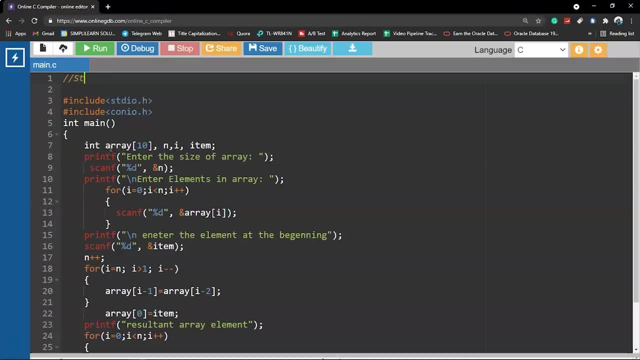 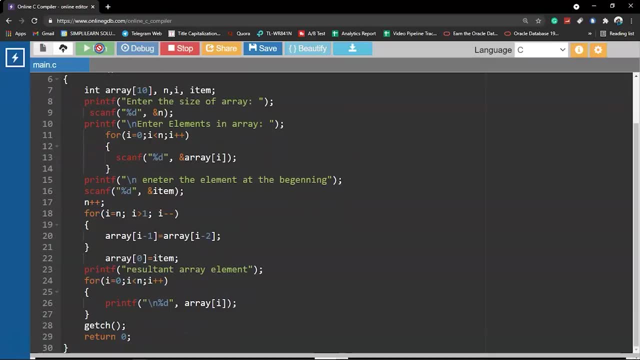 so on my screen you can see an example for inserting an element into the array at the starting position of the array. now let us try to execute this code and see the output. don't worry about the codes. these code documents will be attached in the description box below and you will be able to have an access. 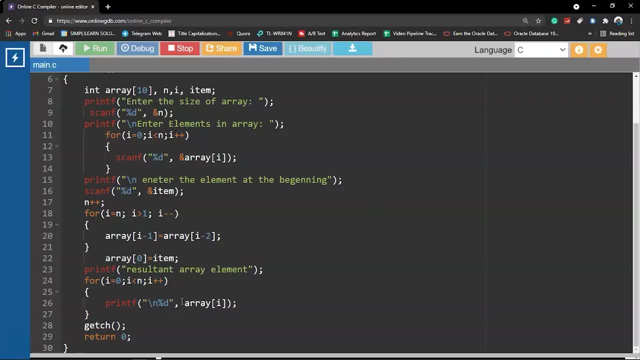 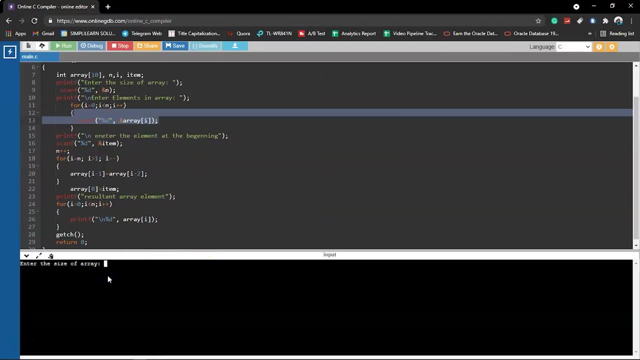 to the code in the description box below and you will be able to have an access to it and run these codes in your personal laptop and get a better learning experience. now you can see the code got successfully executed and now it is asking for the size of the array. let's declare it as 5 and now let's enter the. 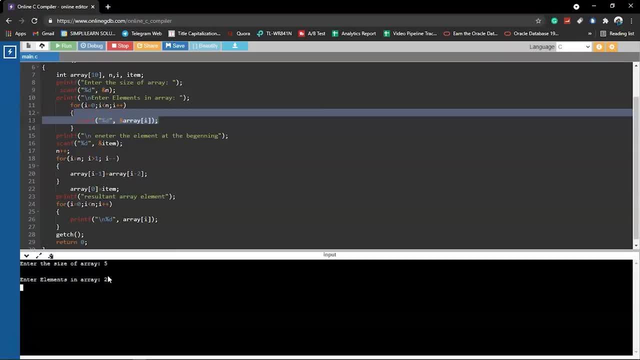 elements into the array. now it is asking for the element to be added at the beginning of the array. now we have two elements that are added at the beginning of the array. now we have two, three, four, five and six existing in the array. let's add the first element one. 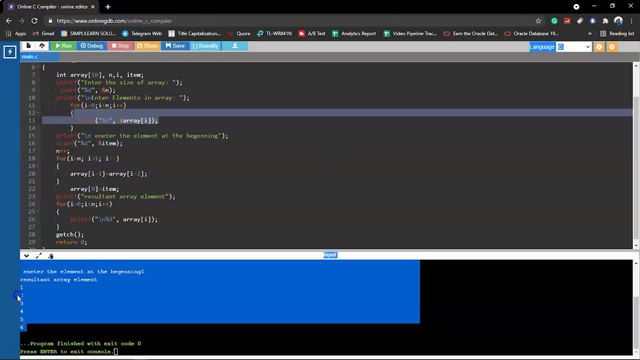 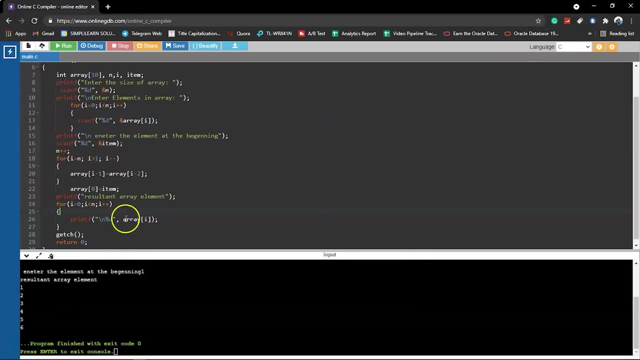 and there you go. the resultant array is one, two, three, four, five and six. the element which we added at the ending, which is one, is supposed to be in the first or the beginning part of the array, which is here at at the first index location, as planned. now let's get started with an other example on the 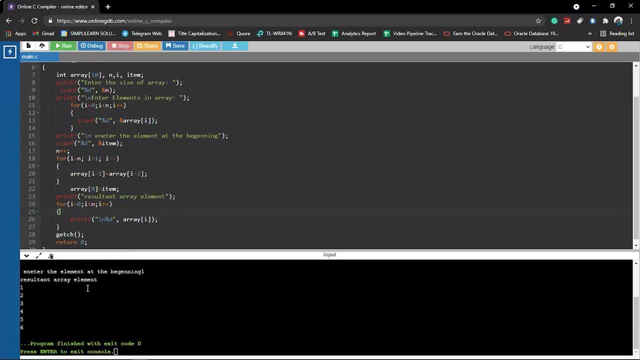 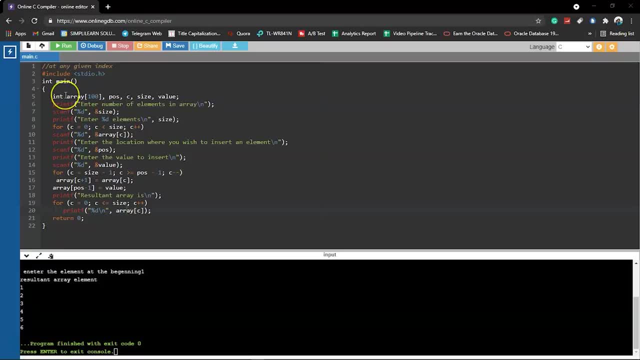 insertion. now let's try to insert an element at any given location, as per the user's choice. so, as you can see, we have a program on my screen and running this program must help us to insert an element into any given location of the array. now let's 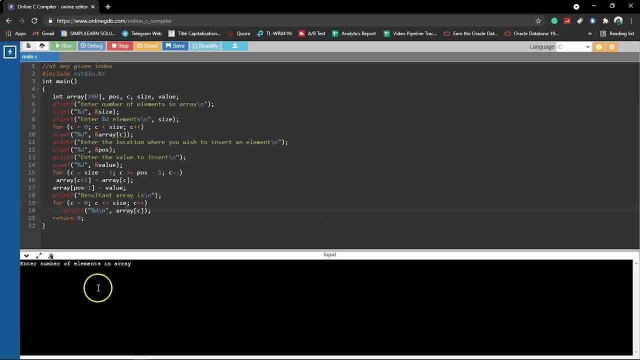 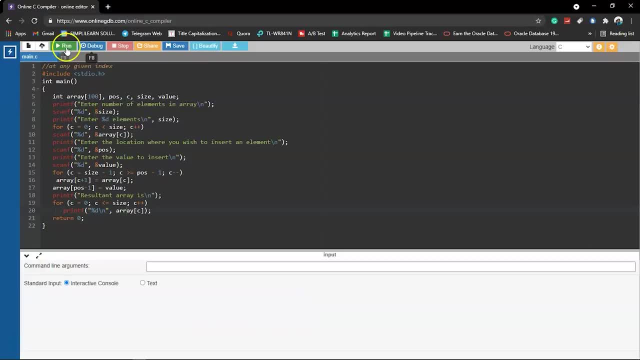 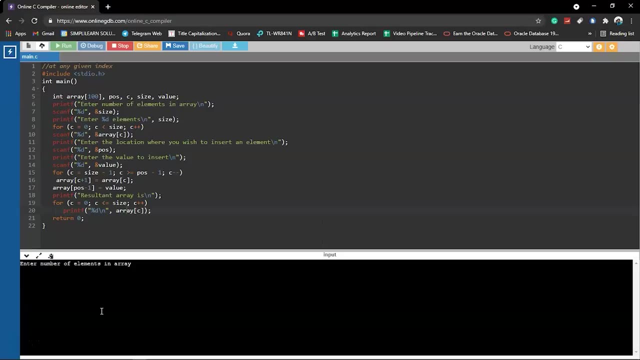 try to quickly run this program and see the output. so there you go. enter the elements into the array. let's enter one, three. let's try to run this program and see the output. so there you go. the program got successfully executed. and now the output is asking for us to be added at the beginning of the array. so let's try to. 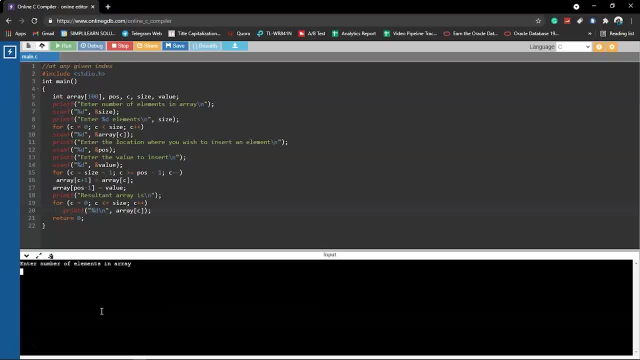 enter the number of elements in an array. now let's say four elements. so now let's enter the four elements: one, three, four, five and six. okay, so the four elements, which is one, three, four, five, are been inserted. now it is asking for the location where you want to insert the element. now let us 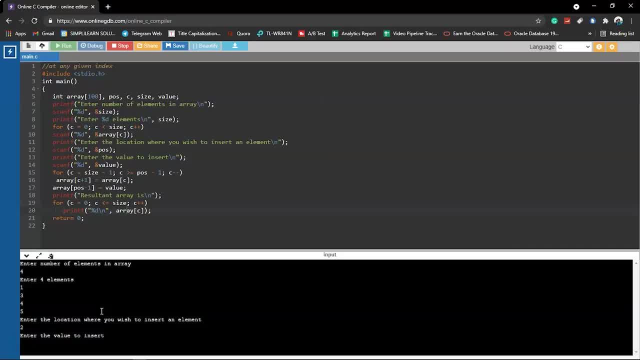 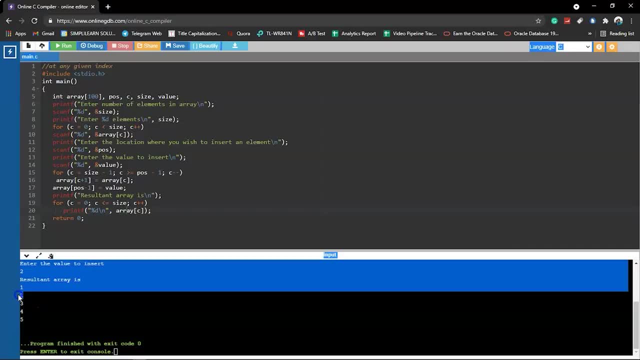 insert it in this second location. now let us set the value as two, and then we'll run this to the next location. Now let us set the value as two, and there you go. the resultant array is one, two, three, four and five, and the element which is two was supposed to be added in the second location, and it has been. 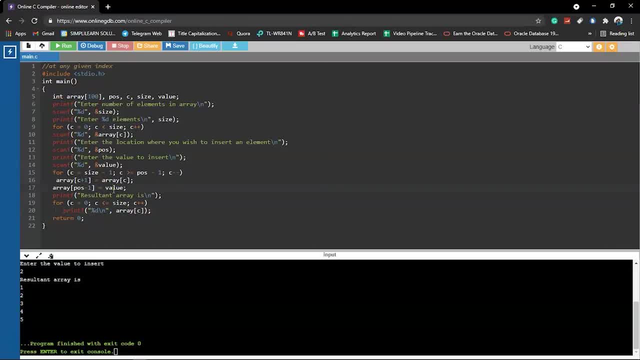 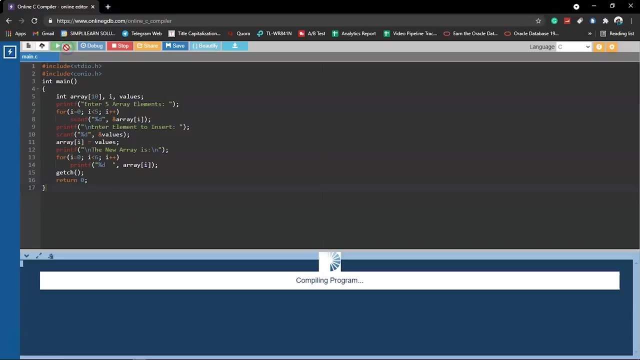 successfully added. now let's try to execute another example based on insertion, where you will try to insert the element in the last position. now this program on my screen will help us to add an element at the end of the array. let's quickly run this program now. it is asking for us to insert the element. 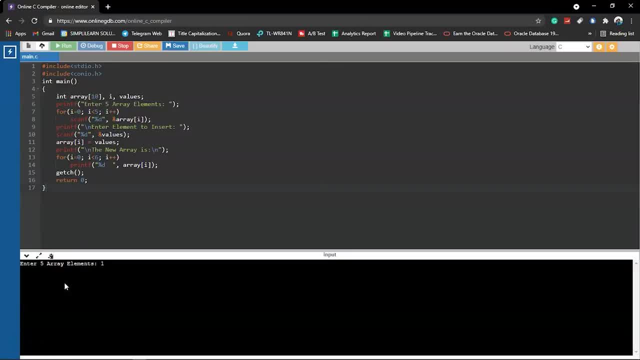 Enter the five elements of the array. Let's enter that Now. it is asking to enter the element to be inserted. Now let us enter the element, and this element should be added at the end location, as discussed. The resultant array is 1,, 3,, 5,. 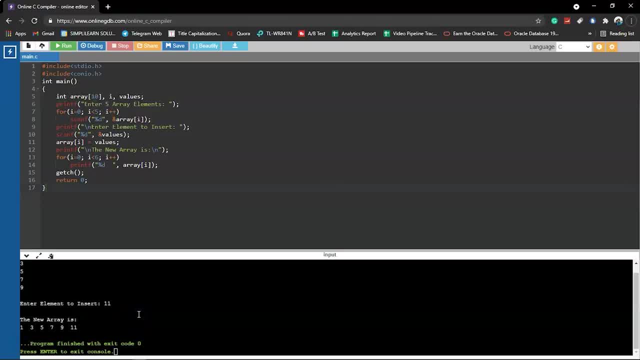 7,, 9 and 11.. Now let's continue with the deletion operation. Now the program on my screen is an example for deleting an element from the beginning position of an array. Now the program got successfully executed and it's asking for us to enter the size of the array. Let's enter the size as 5.. 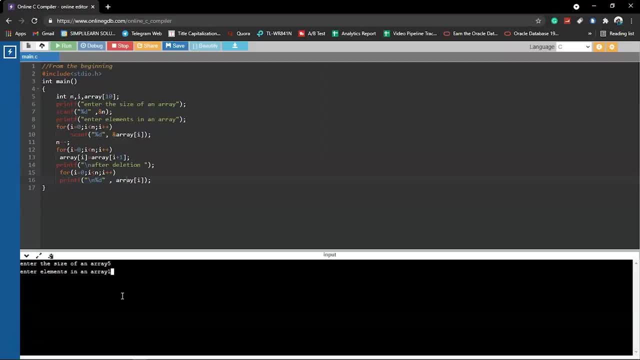 And now let's enter the elements of the array, that is 1,, 2,, 3,, 4 and 5.. Now the element from the first location, that is 1, has been deleted and the resultant array is 2,, 3,, 4 and 5.. Now the code on my screen will help you to. 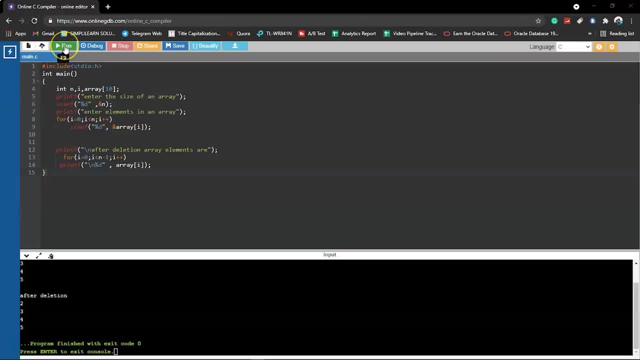 eliminate the element from the ending location of an array. Now let's try to quickly run this program and see the output, So you can see that the program is successfully run and it is asking for us to enter the size of the array. Let's enter 4.. Now let's enter the elements of the array, that is, 1,, 2,, 3,. 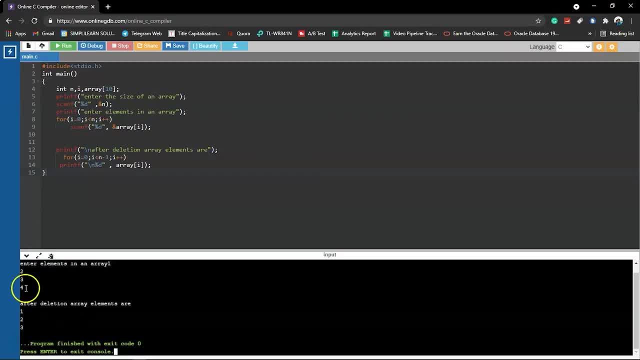 and 4.. Now, after eliminating the last element from the array, that is 4,, we have the resultant array that is 1,, 2 and 3.. Now a little homework for you guys. Let's try to execute an example for deleting an element from any location of an array. This will be a homework. 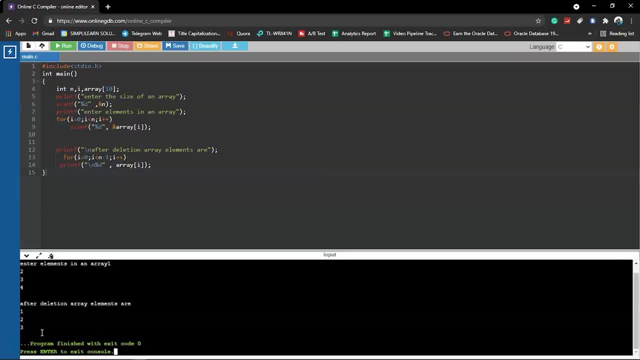 Now, don't worry, try on your own, and if you don't get that, you can refer to the comment sections below, where you have the code document attached in the description box and you can refer to it. Now let's try to execute an example for deleting an element from any location of an array. 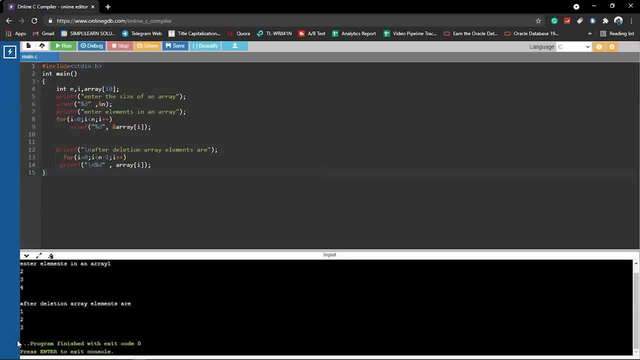 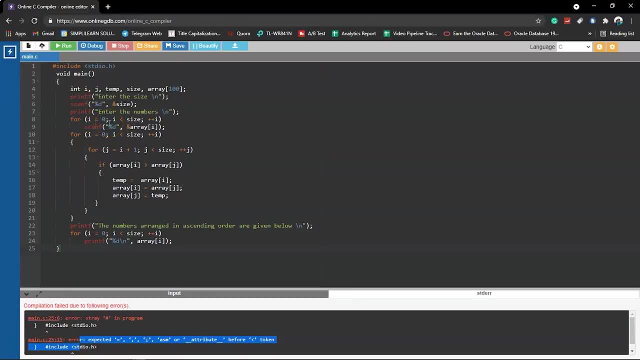 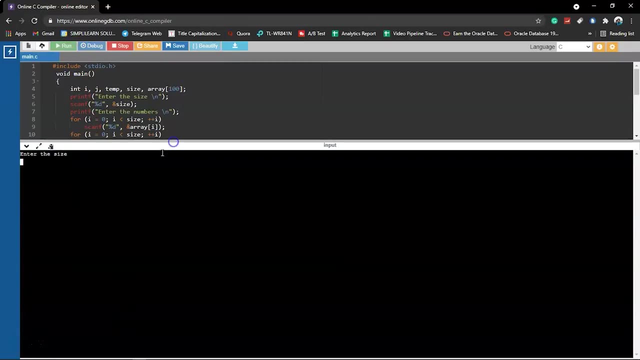 Now let's continue with the next operation, where we will search for a given element in the array. So you can see that on my screen we have an example which will help us to sort the elements in an array. Let's quickly run this. So there you go: the program got successfully executed, and now? 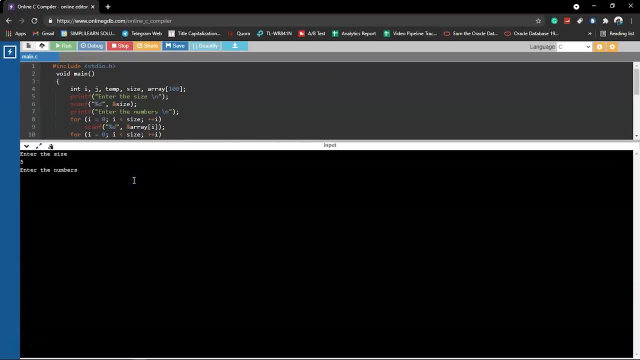 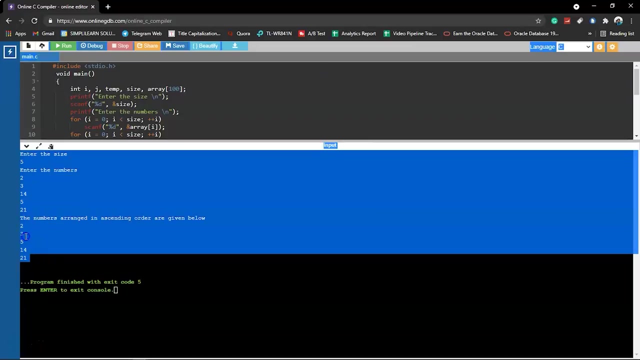 it's asking for the array size. Let's enter 5, and now let's enter the elements in a random order. So once again we have the resultant array. so the array should now be sorted. So there you go. the array, after being sorted, is 23514 and 21.. So there you go, the array. 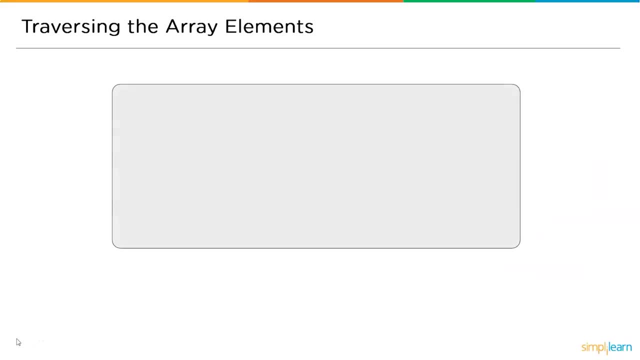 got sorted. So now we have finished our practical session, Let's have a quick overview again. So traversal in an array is a process of visiting each element once. Traversal can be done by various means, that is, by counting the array elements, printing the values sorted in the arrays and some of all elements present in the array, and many more. 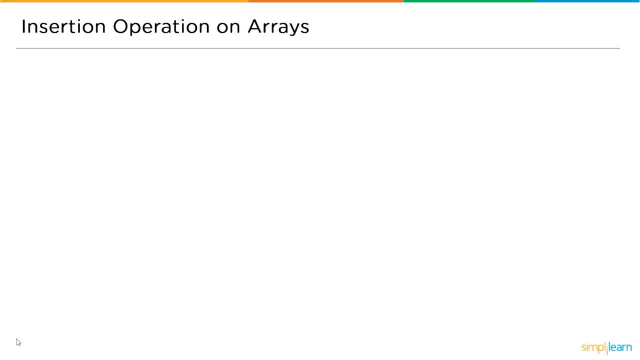 So this is how we traverse our array from the first location to the last location. Again, the insertion operation. Insertion in an array is the process of including one or more elements in an array, and it can be done at the beginning, at the end and at any given. 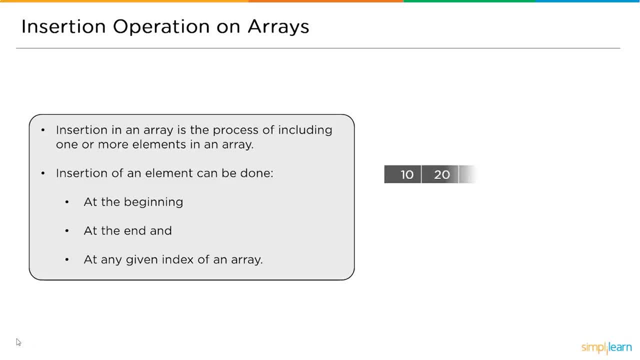 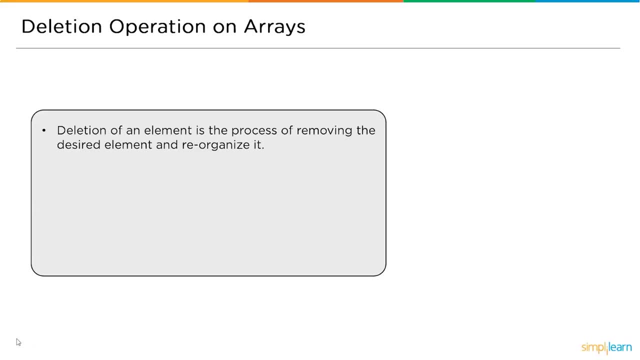 index of an array which we executed for all the three types of examples Now. next, we have the deletion operation. So deletion operation, or deletion of an element, is a process of removing a desired element and reorganizing the array, and it can be done at: 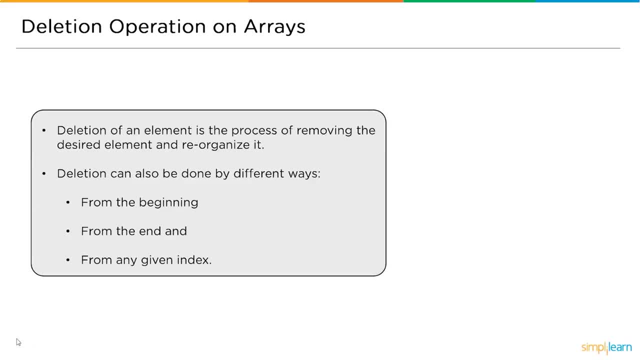 the beginning, at the end and at any given index. So we have executed the example for at the beginning and at the end and the homework was at the given index. Don't worry, if you don't figure it out, you can always refer to the example document which is mentioned in the description box below. 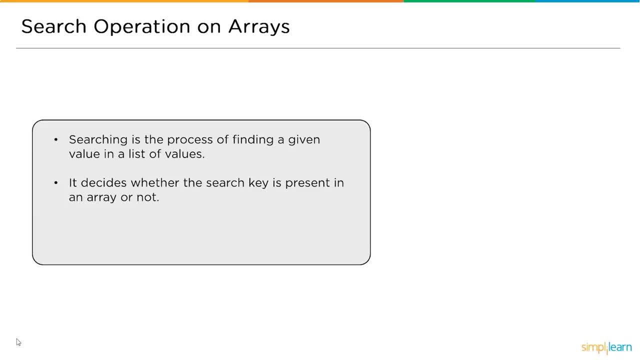 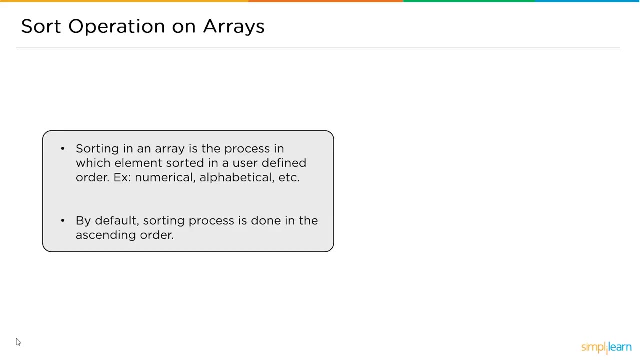 Now the search option. Searching is a process of finding a given value in the list of values and it decides whether the search key is present in the array or not, and we have executed an example on that. And again, the sort operation, where we will sort the given array If the given 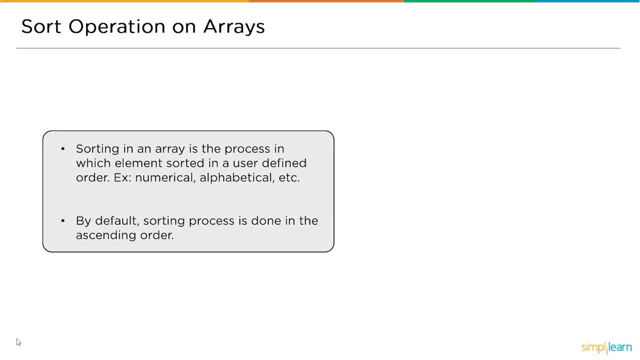 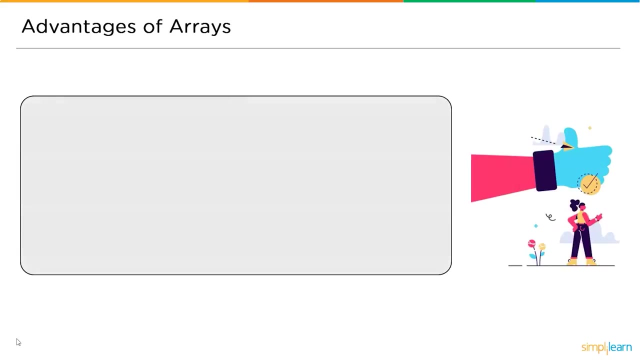 array is not in the default order or in a given order that is ascending or descending, then we can sort the order of the array by the user's choice, given it is ascending order or descending order. Now, in the next section of the tutorial, we will discuss the advantages of using arrays. 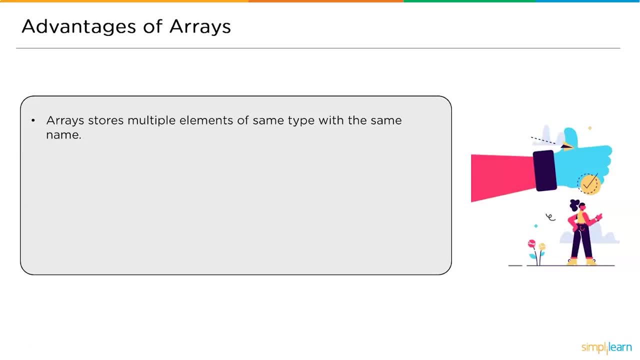 So the first one is: array stores multiple elements of same data type with same name. Next one: elements in an array can be accessed randomly using just the index number Array. memory is predefined, so there is no extra memory loss. Array avoids memory overflow. And finally, 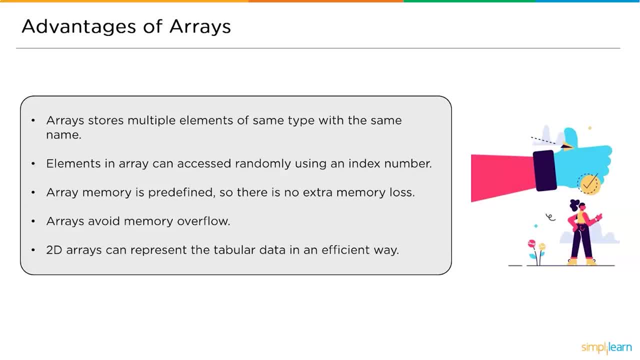 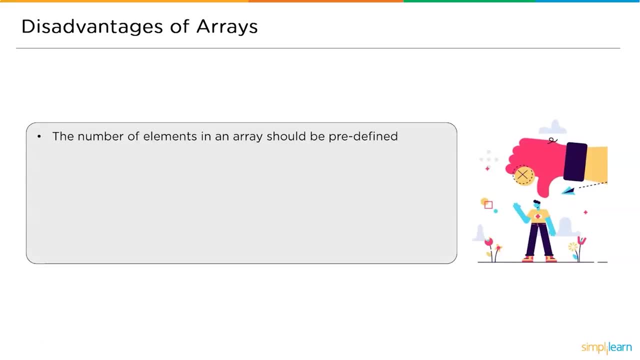 2D. arrays can represent the tabular form of data in a very efficient way. Now let us also have a look on some of the disadvantages of using arrays. The first one: the number of elements in an array should be always predefined, So there is no chance. 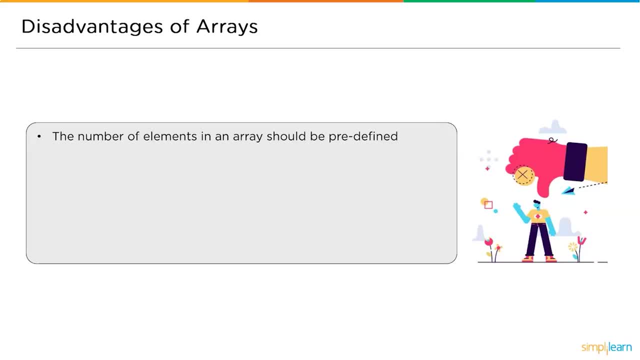 that you can add some extra element in the last moment. Array is static in nature, so its size cannot be varied after declaration. What if? consider that you wanted to store 10 student data in an array and you end up having just 7 students? so the remaining 3 is a waste right? So you are?